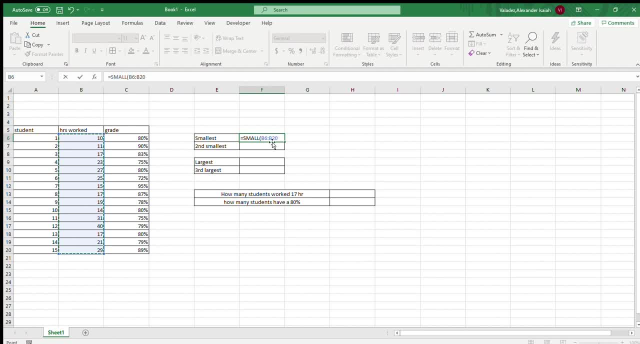 So that'll be cell B6 and B20, and, as you can see, I've entered that in there and then I'm going to do comma and we want to find the smallest one, so we're going to put 1.. Once we have that, we're going to click enter, and so the smallest number in here happens to be at top, which is 10.. Alright, so if we're looking for the second smallest, we're going to do something very similar. 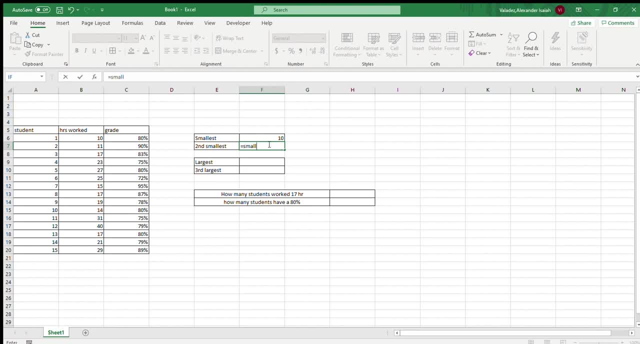 We're going to put equals small and then put the parenthesis, and then we're going to do the same array, but if we want to find the second one, we're going to put comma 2, because we want to find the second smallest number. If we wanted to find the third smallest number, we'd put 3, but for this we want to find the second, so we're going to put 2,, click enter and it happens to be the second number, which is 11.. 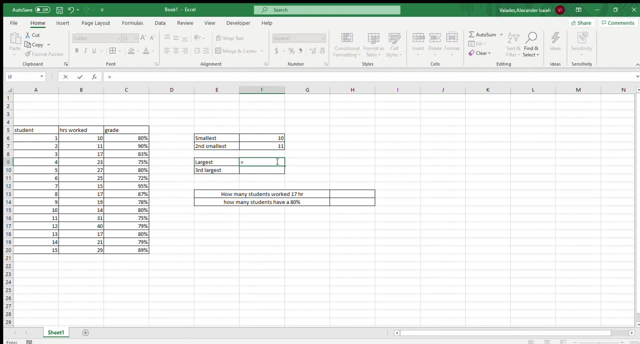 We're going to look for the largest. it's going to be very similar. we're going to put enter large, we're going to click the dataset highlight all the way down, alright. and then we want the first largest number, so we're going to put 1, that happens to be 40 in this given dataset. 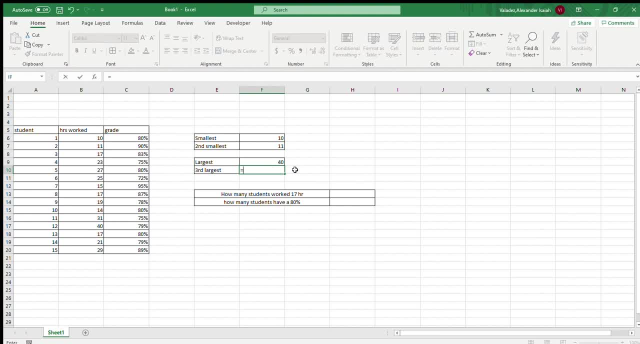 Alright, now we want the third largest number, so we're going to put enter equals large. type that out right there. Like I said, when you're in your Excel document, you're going to be able just to type it, and then it will. there will be a little pop-down bar and you can just click that. If not, you can always just type it this way and it will do the same. 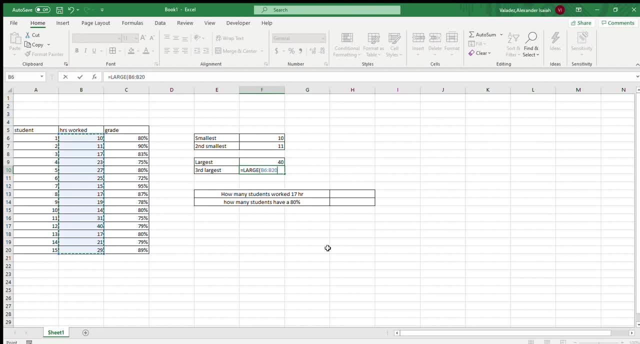 So we're looking for the third largest function. we click the data, all the data that we're trying to sort through. we're going to put comma. since we want the third largest, we're going to put 3.. If we wanted the fourth largest, we'd put 4.. 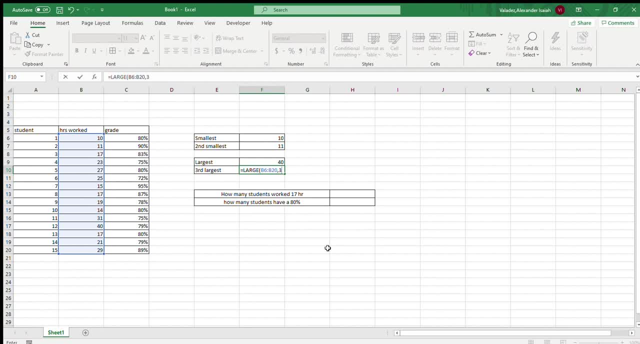 If we wanted the fifth largest, we'd put 3.. If we wanted the sixth largest, we'd put 5, so on and so forth. Alright, so the third largest number in this dataset of hours worked is going to be 29.. 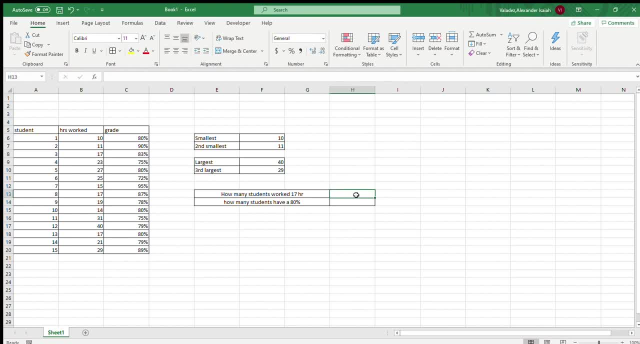 Alright. Alright, so for this question we are going to use the COUNTIF function. So the way that works is: we have a question here that says how many students worked 17 hours, alright. So instead of going through this data and counting each time we see 17,, we can put enter. 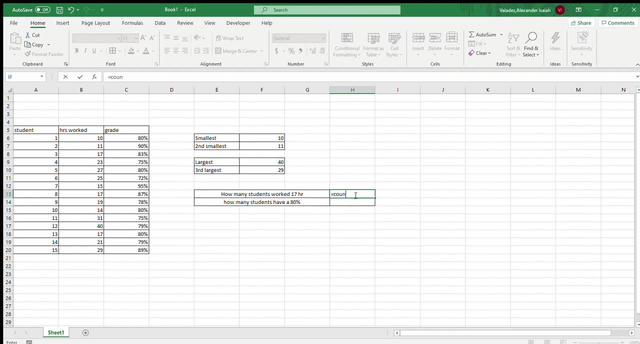 We can type in COUNTIF: Alright. So then we're going to highlight the given range that we're looking. Alright, so that's b6 through b20.. We're going to put comma and then we're going to give what we want them to count. 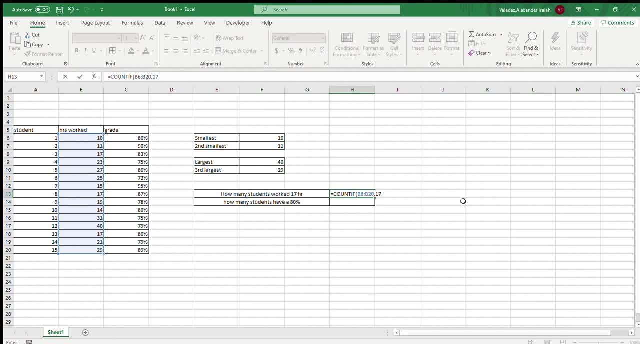 So we're going to want them to count for anyone who has worked 17 hours. so we put that 17 in and then we click Enter. So there's three people. We have worked 17 hours and we can just verify 1,, 2,, 3.. 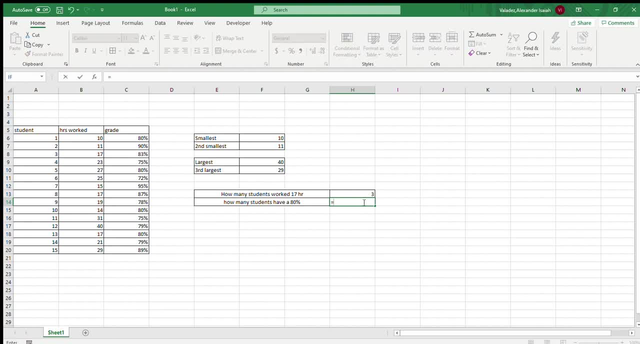 Yep, that is correct, All right. same thing for this question: How many students have an 80% in the class? All right, and then we're going to press equals count, if. All right, and we're going to highlight the given range that we're trying to sift through. 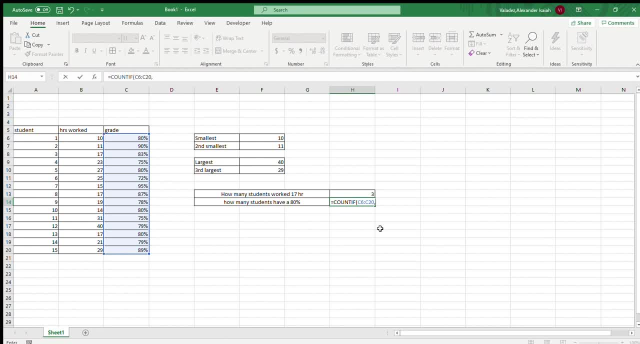 and we're looking for 80%. So I'm going to put 80, and I'm going to make sure to incorporate that percent sign as well. If you don't incorporate that, then you'll have some problems And then press enter and then you're good to go. 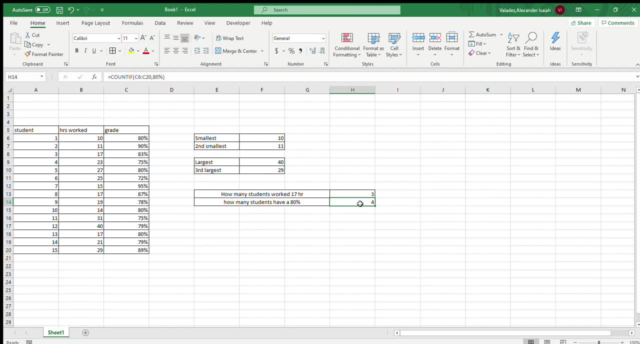 So right here I'll just click back up here- That's how many students we used the count if function You can see up here. it tells you exactly what we put in to get that. So we put count if C6 through C20.. 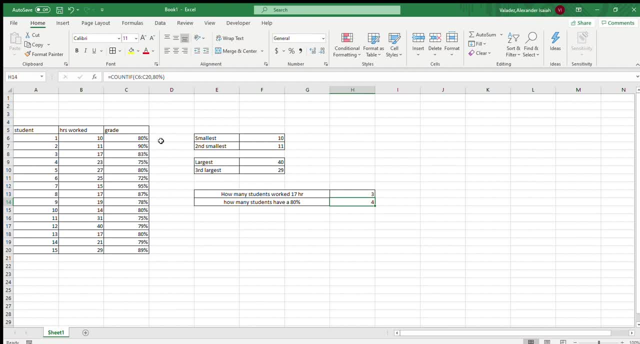 If it's 80%. So there are four 80%s in here, And while this data is easy to just take a look at and kind of count on your own, you may be like, well, why would I even use that, if it's just easier to count? 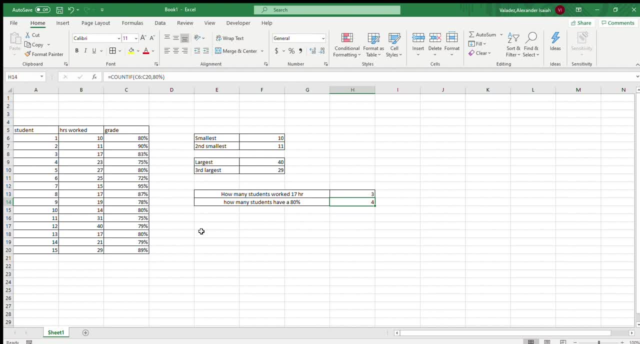 There's going to be certain times when you have 100 plus data points and it's easier just to use this function, So that's why we use that. All right, then we can look in here. For this one. we did the count if 17, B6 through B20..